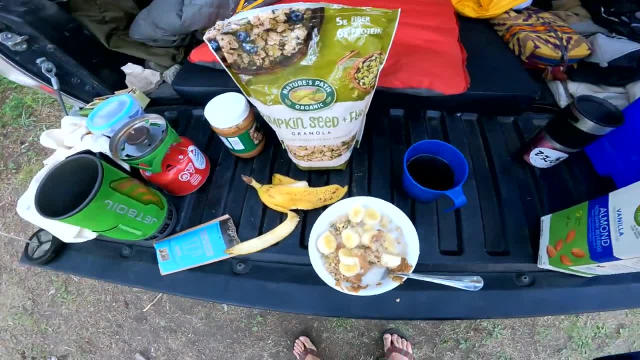 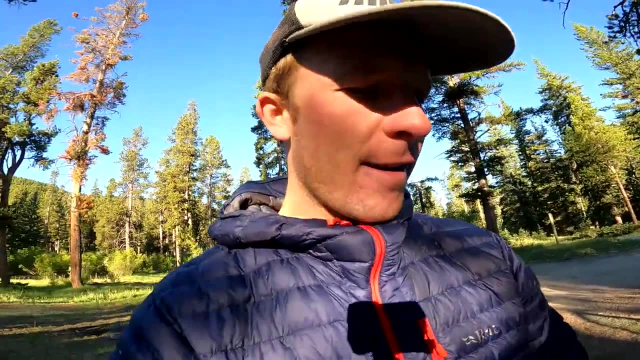 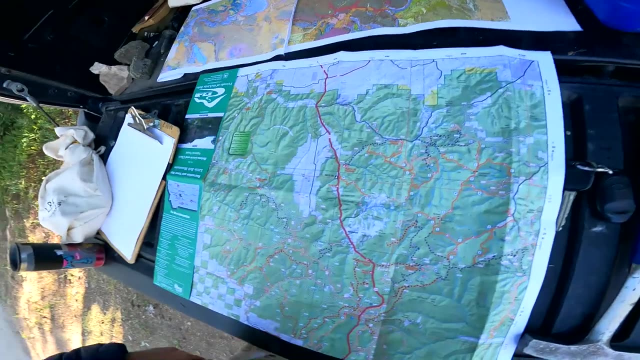 the field. You know peanut butter, some granola, banana, a little bit of almond milk out here. All right, the morning is moving. The plan is kind of made. I kind of made a plan last night, honestly, but I'll show you guys what we're working with here. Looking at a couple maps: 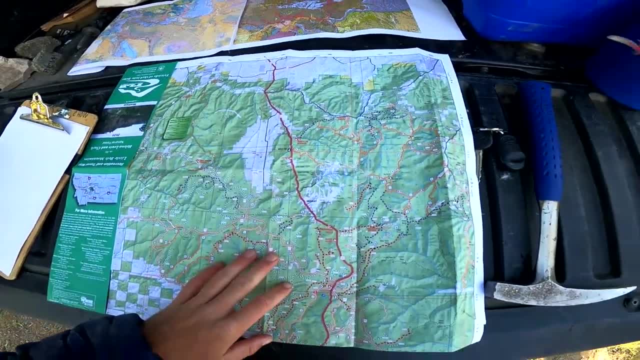 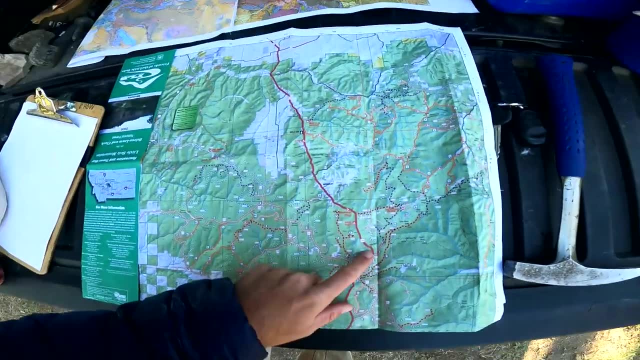 This is just a Forest Service map that has you know roads and you know trails. Right now we're up Jefferson Creek, which is right up in this region. This is one of the main roads that comes right through the center of the Little Belt Mountains. 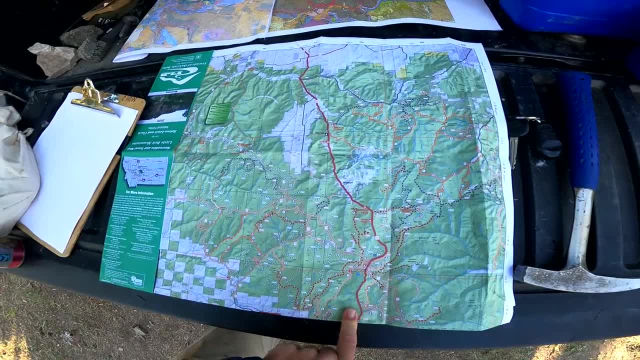 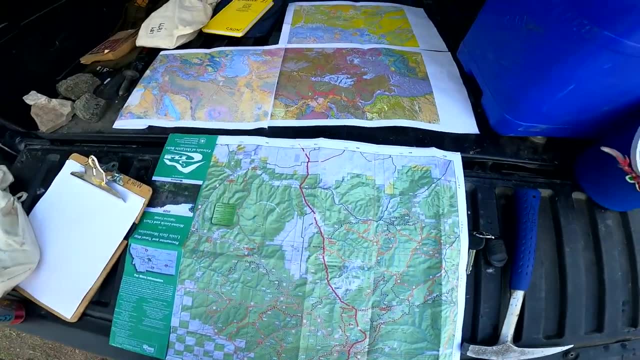 And the first thing we're going to do today is go up the high point in the range which is called Big Baldy Mountain. It's right here. I think it's going to be about 10 or 12 miles a round trip, And up here we have the geologic map or some of the 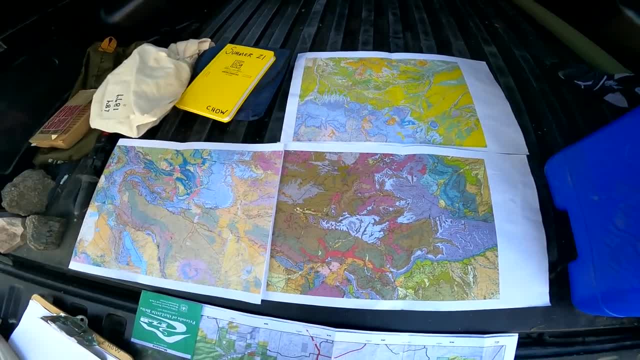 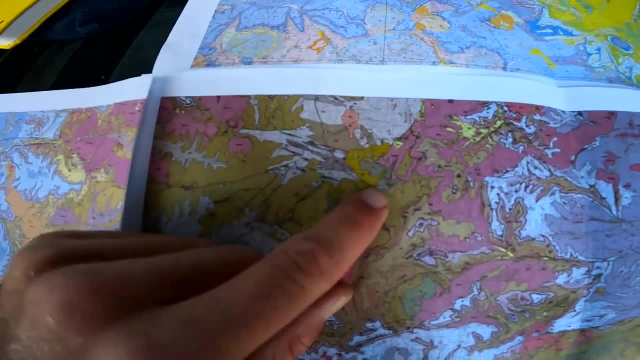 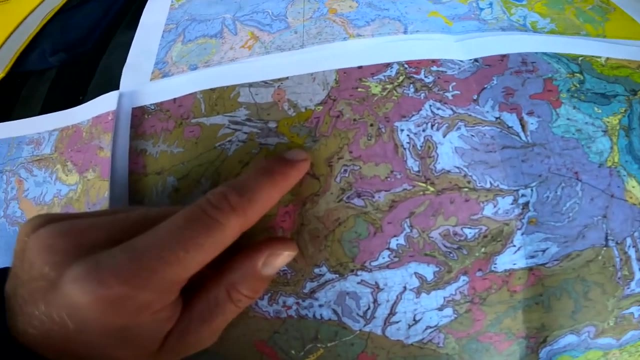 100,000 scale geologic maps of the Little Belt Mountains. Basically, that same highway meanders its way up through the range. here We are parked in this region near a rock formation called the Nyhart Quartzite. Quite interesting and important, But what we're going to do is jaunt at Big Baldy. 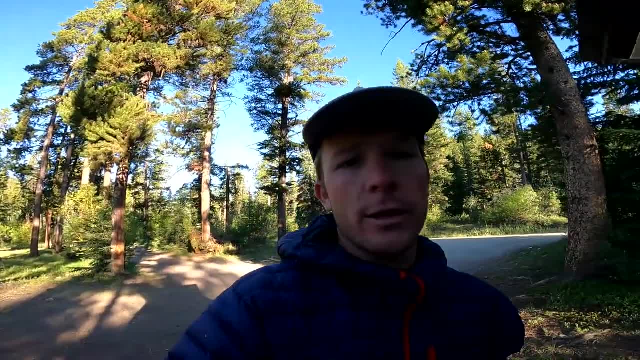 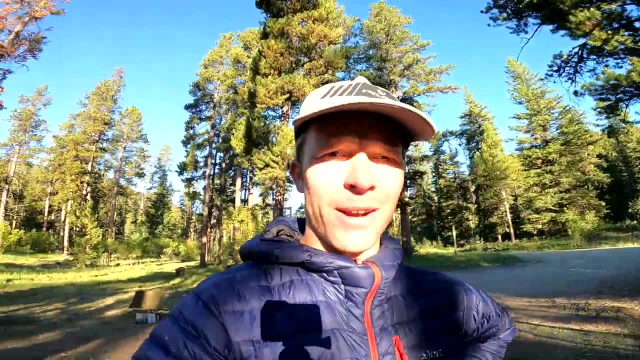 which is up in this region- It's kind of how the day usually starts- is looking at some maps, kind of getting oriented, And we're going to go up there, We're going to get a nice view and maybe do a little bit of geologic mapping. 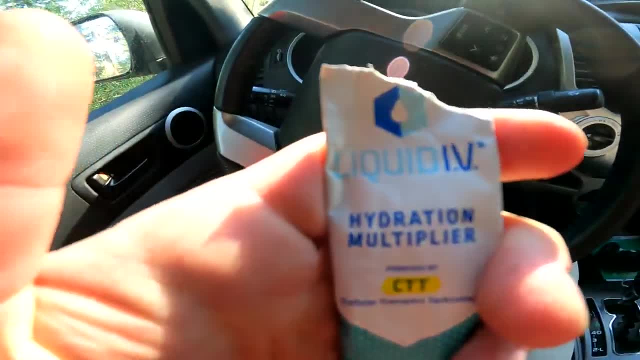 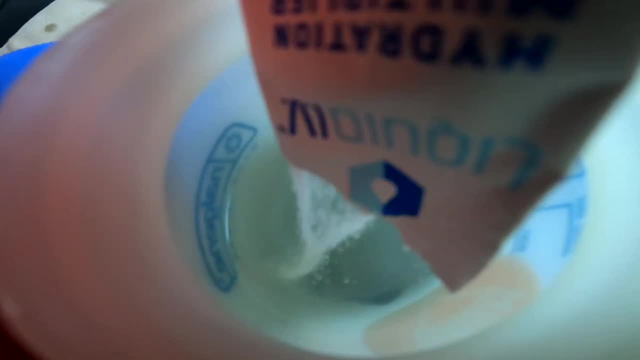 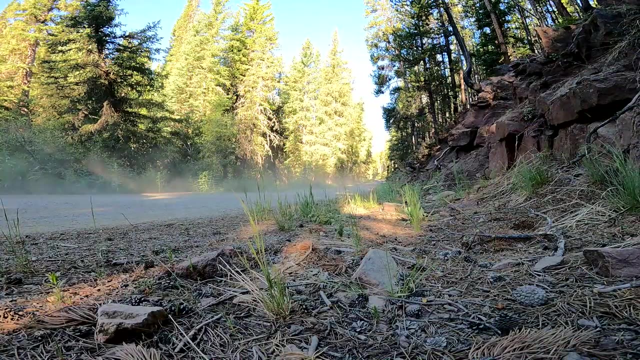 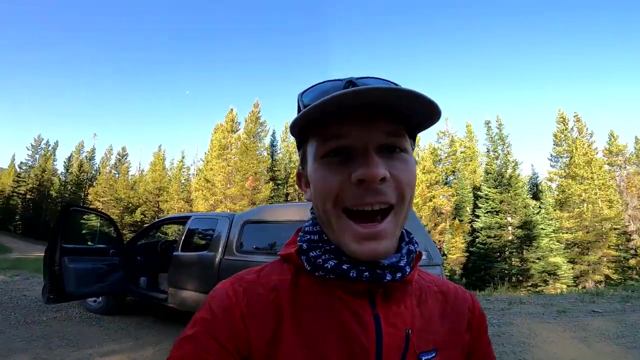 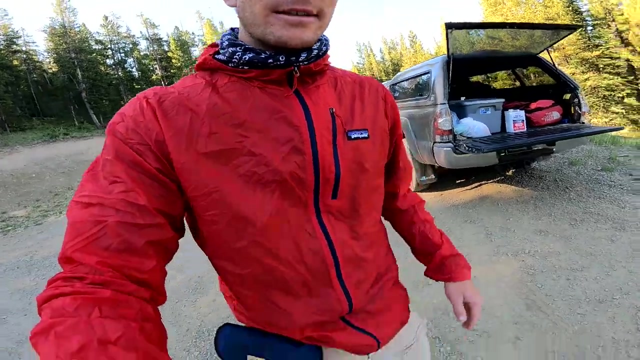 Cruising right along, Liquid IV highly recommend. Even when you're in the field alone, it's very important to swag out heavy. Got the you know just some Smith Shades. Always got to have the buff Patagonia Windbreaker, Some ragged-ass Carharts. 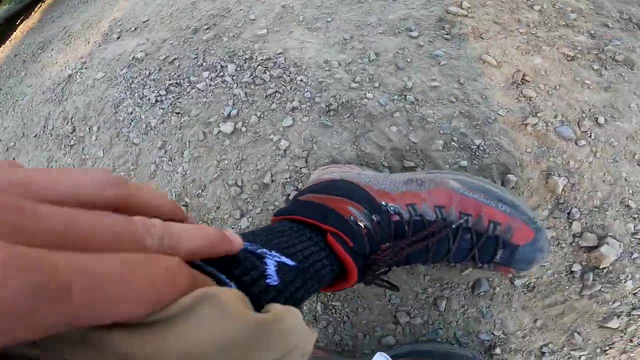 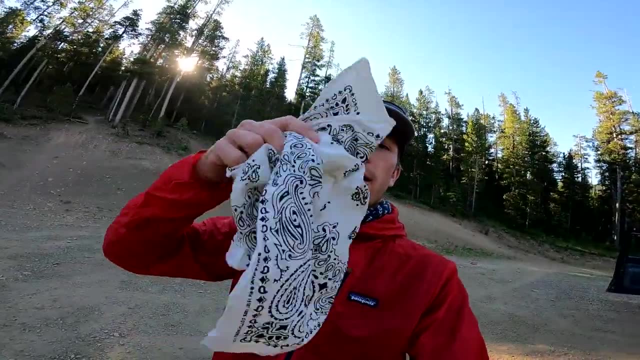 Ragged, La Sportivas Rock, the Long Sox, Puma, Not the best You know, just a shirt underneath, tucked in Bandanas, crucial piece, Great to fit 1 to 10.. Oh, Plateau Designs too. 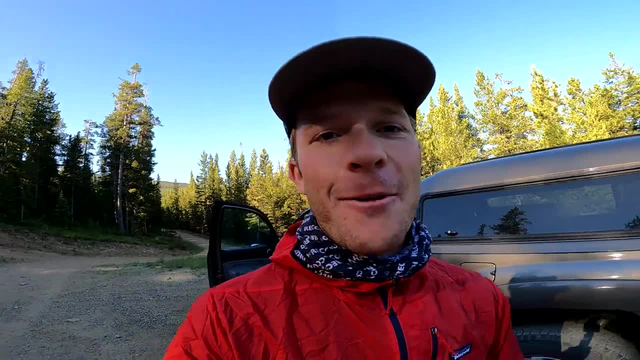 Drop it in the comments. Time to do the warm up. Always got to warm up before a day in the field, so I'm gonna, you know, get the heart going a little bit And then we'll get on the trail. 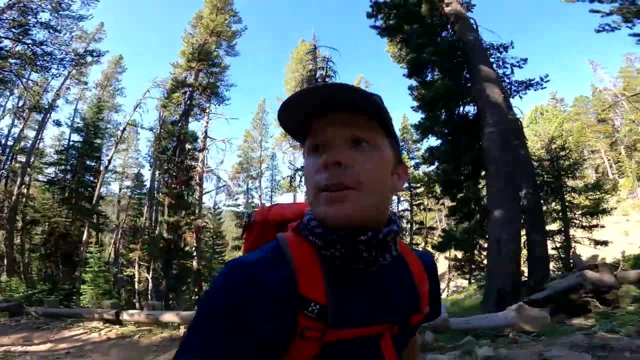 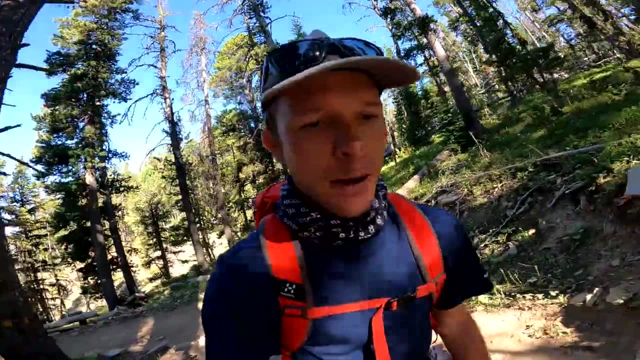 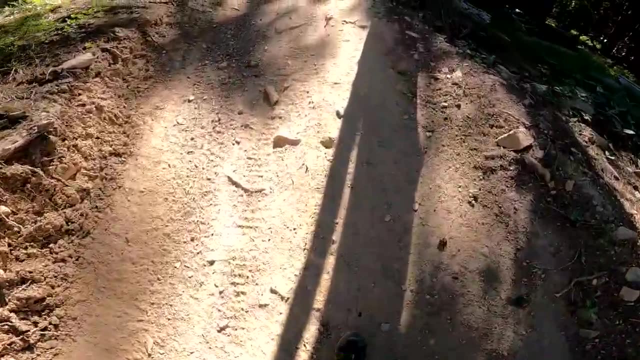 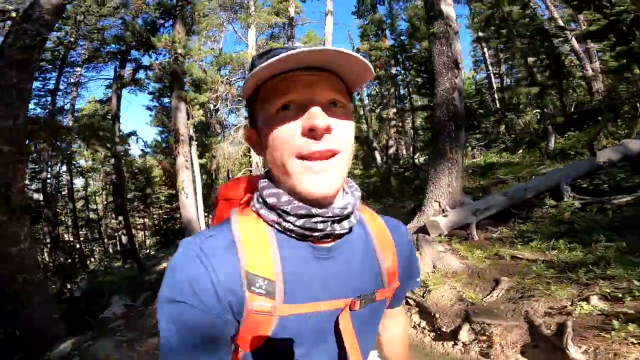 I've been hiking about 35 minutes minutes, just about just over two miles up this little trail. um saw a couple deer, pretty chill morning so far been following their tracks uh, in this really dusty, uh pretty well established trail that motorcycles almost certainly use, but we're cruising the little belt mountains. 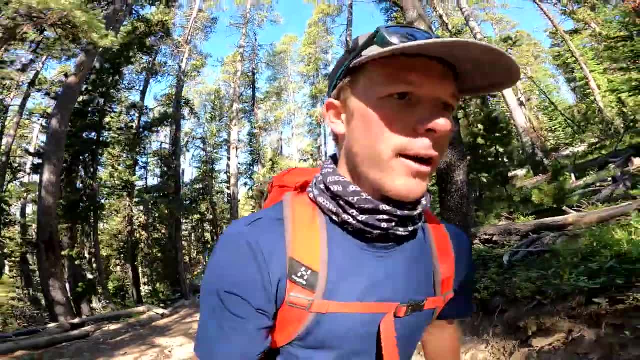 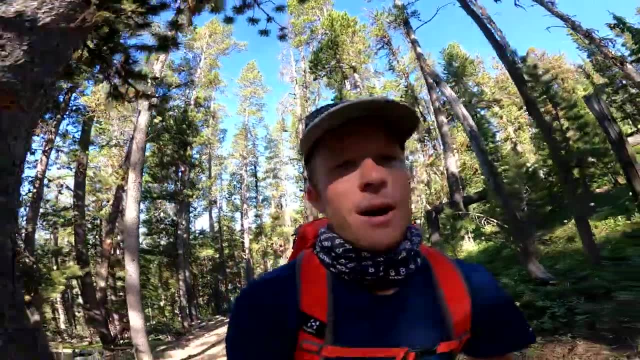 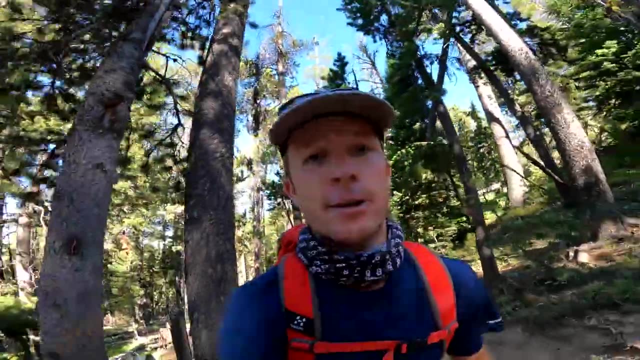 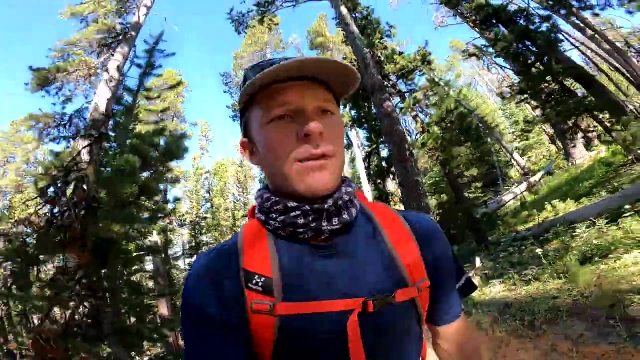 densely forested. it's one one of the reasons that geology- doing field geology here- is a challenge- is because it can be can be hard to find outcrop exposed. but i have a hunch that, due to the elevation of this peak that we're going up, we'll get some nice views of the range and that's kind. 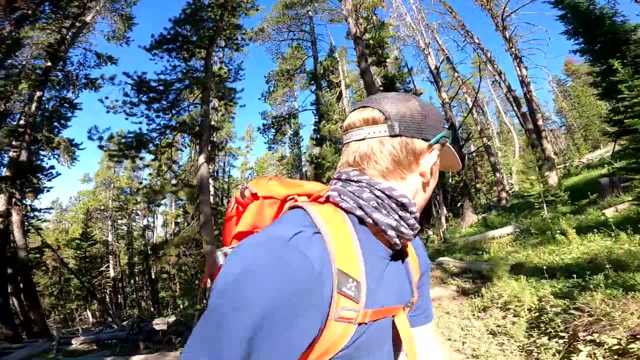 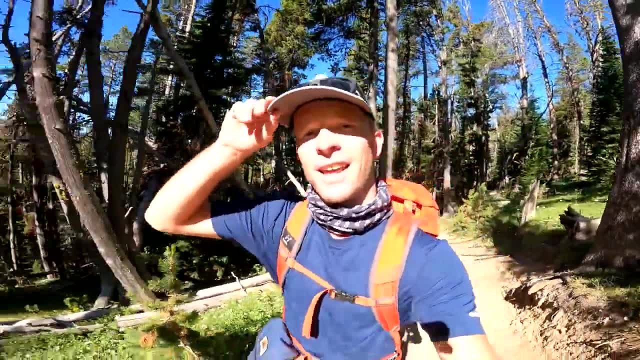 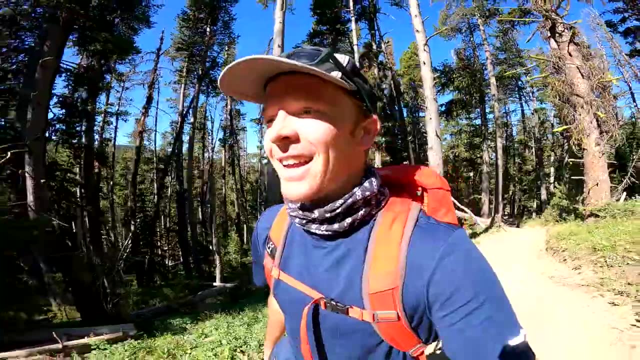 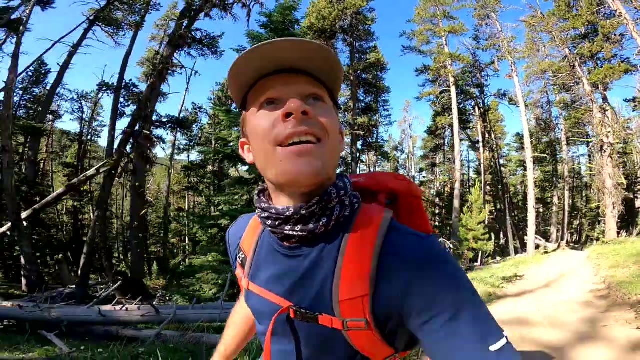 of the purpose of today's uh morning is to get some perspective learned early on. doing geology that um, it pays to get up high as early as possible. even though i have a generally good idea of the topography and the the local geology, it'll be good to to get high. but here's the general 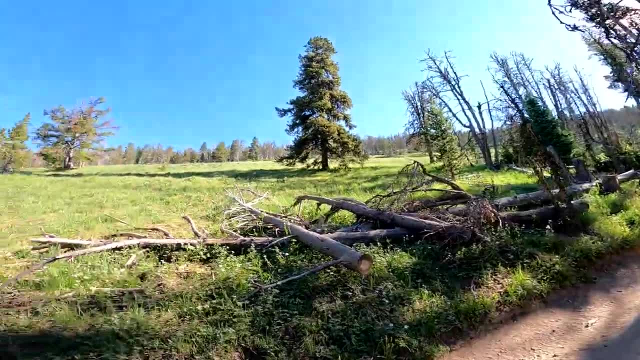 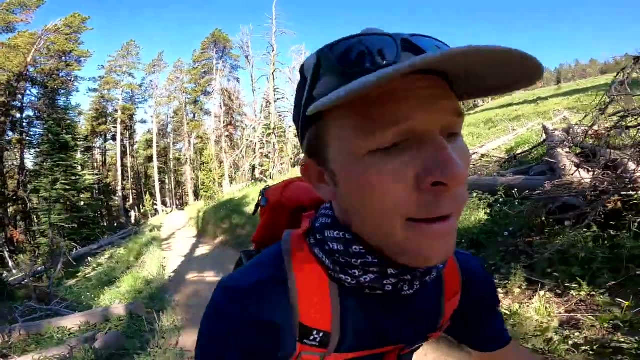 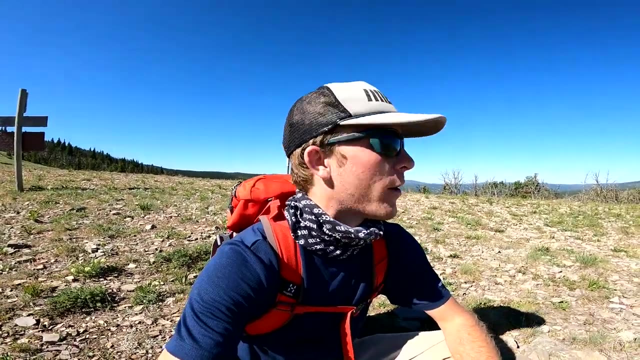 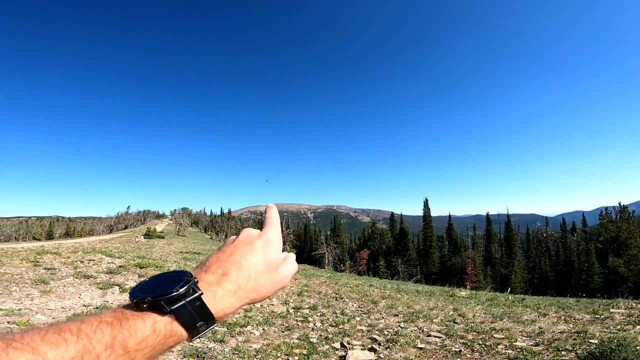 trail. you know, really dense lodgepole pines open up a bit above me, um, but we'll get up there soon enough and show you around. all right, everybody just gained about 1300 vertical up on a little saddle. what a beautiful day. it's getting kind of hot, but our destination is: are those broad peaks over there? um, it might. 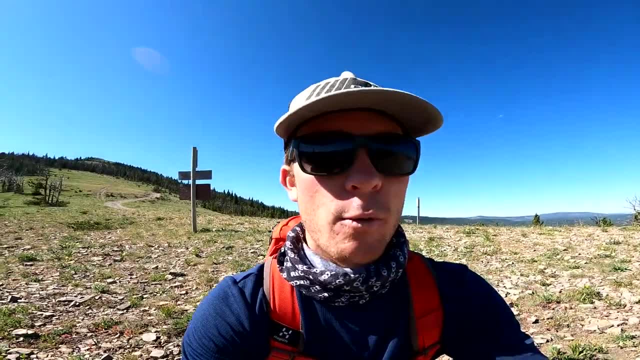 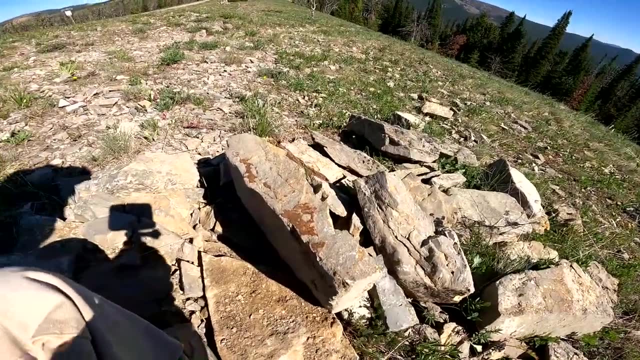 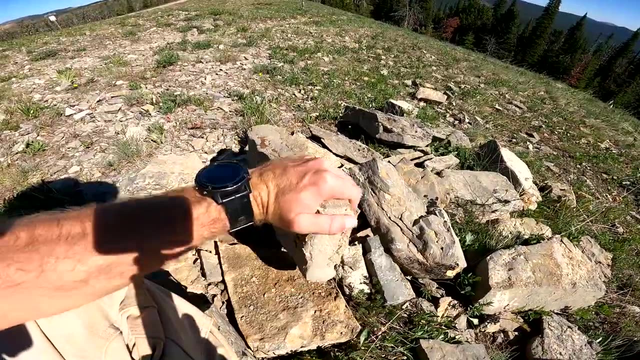 be kind of long, but it's very easy walking, so it's going to be worth it. um, i wanted to show you an example of, you know, coming across a rock in the field right away. having worked in Montana and being familiar with the geology of the western US, I know that this is paleozoic passive margin. 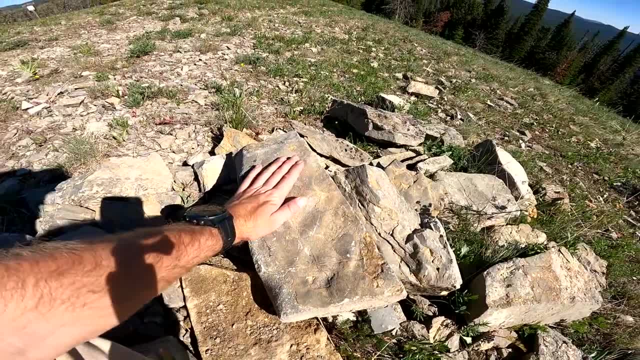 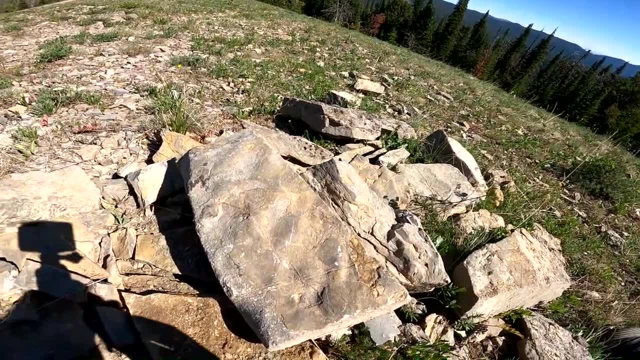 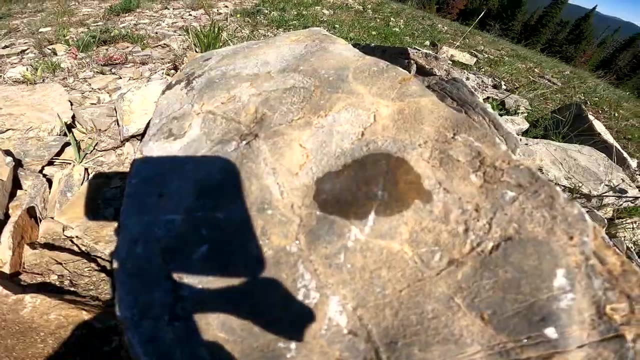 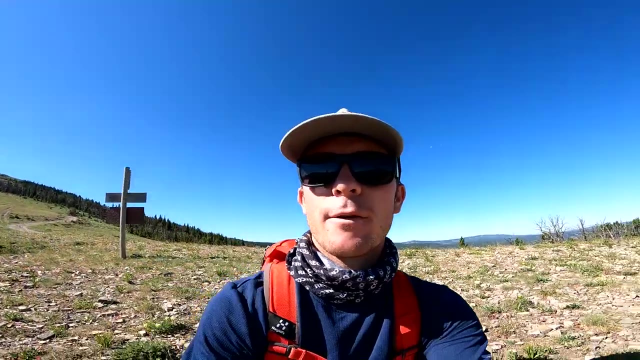 strata. this is limestone. it's known as the Madison limestone up here in Montana, so you can tell right away as a geologist that this is limestone, based on just the look, basically. but we do have tools. if you can see that fizzing there, it's a bottle of hydrochloric acid, pretty dilute but it reacts. 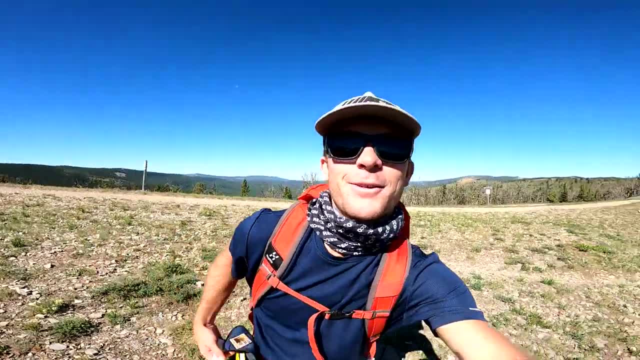 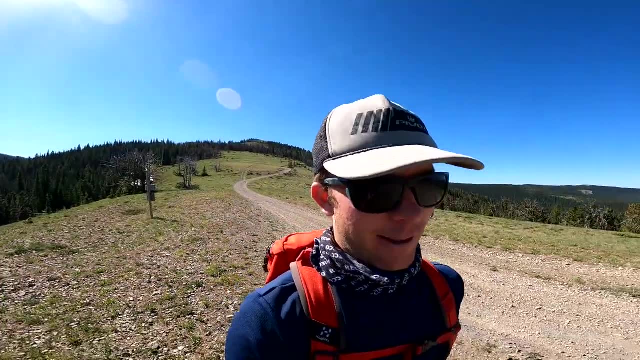 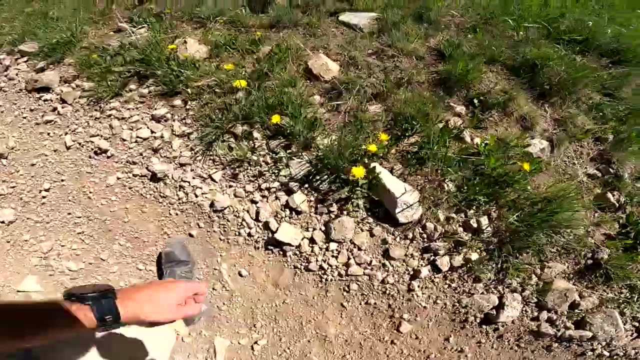 with calcium carbonate, CaCO3, which is what limestone is made out of. so there's some field geology for you, but we're going to keep cruising just a little bit of limestone. nothing to write home about, but yeah, we're moving right along. in places like the little belts, you need to pay a lot. 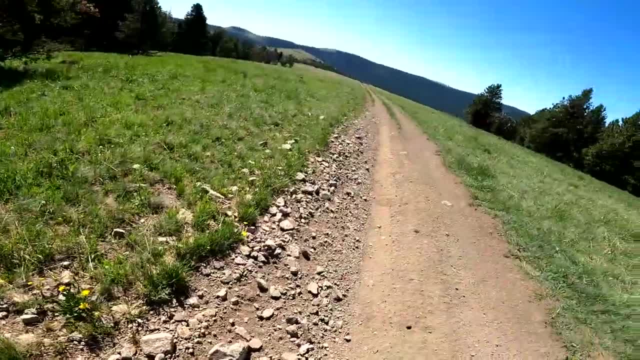 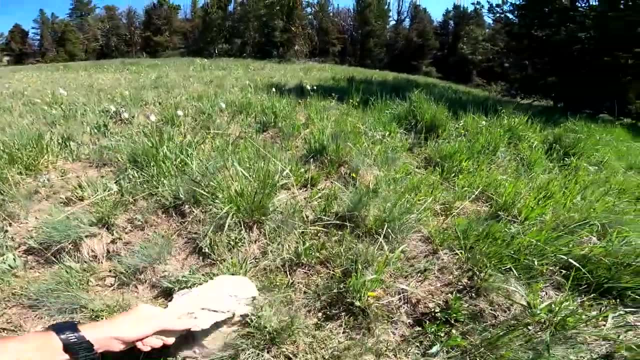 of attention to the float, which is these rocks that are just, you know, along the side of the road, maybe scattered as boulders, uh, in the fields. but you know, I've been walking through, oh, rock hammer's in my backpack, uh, I've been walking through all this. 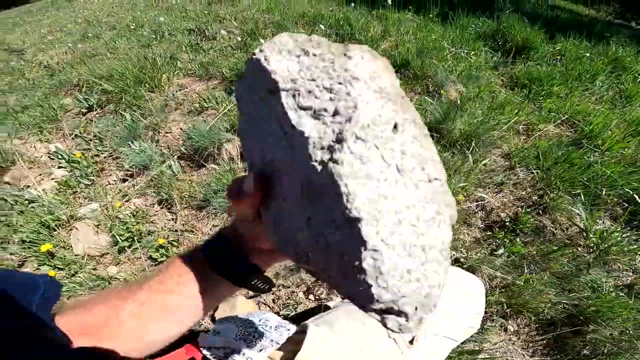 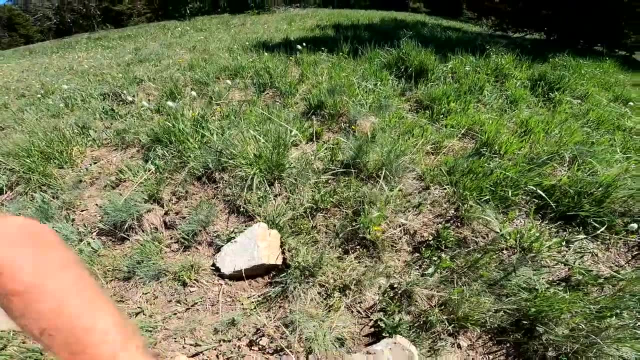 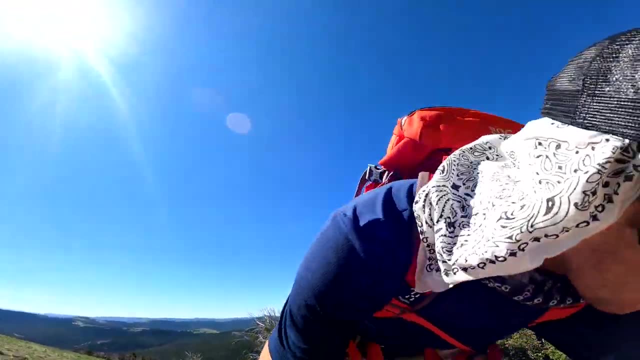 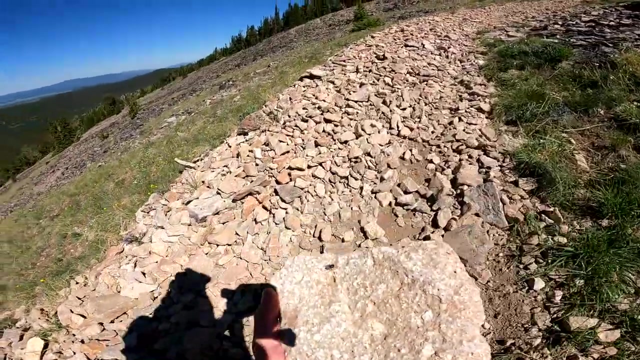 limestone down there, and all of a sudden, we come across this, uh, this beautiful granite, um, which makes sense. obviously, the mountain I'm about to climb up is made entirely of this stuff. well, walking up now, walking through an assortment of intrusive igneous rocks, we've got some andesites, some granodiorites, some 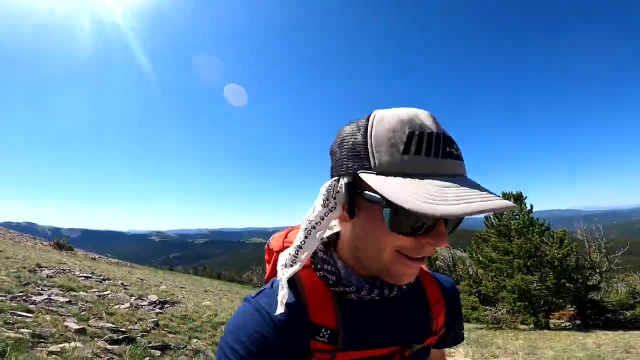 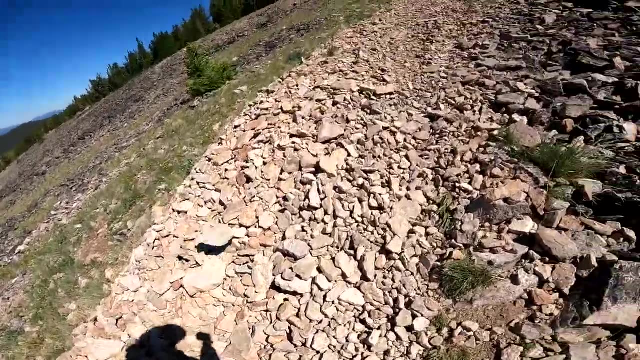 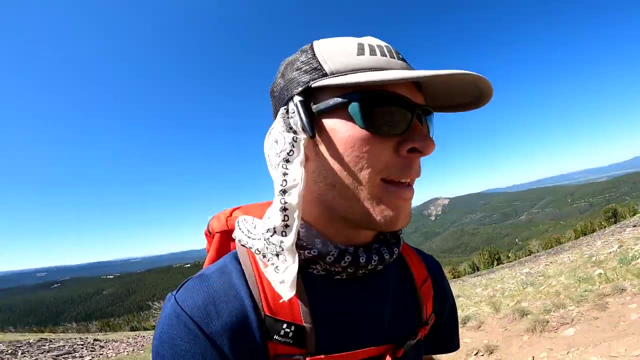 borderline rhyolites. um a lot of words, I know, but you can see, in a lot of these rocks, big plagioclase, phenocrysts, uh, keeping an eye on the textures, hearts, hearts beaten. it's 140, we're cruising. see at the top, son. 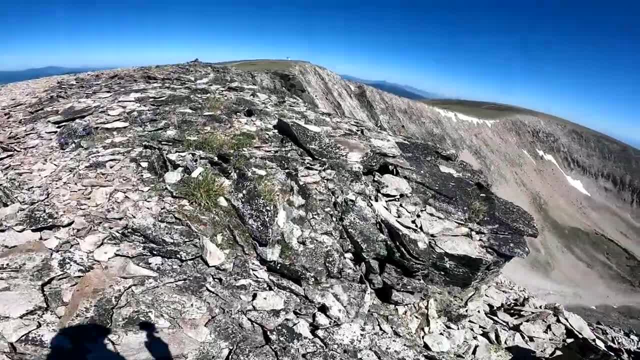 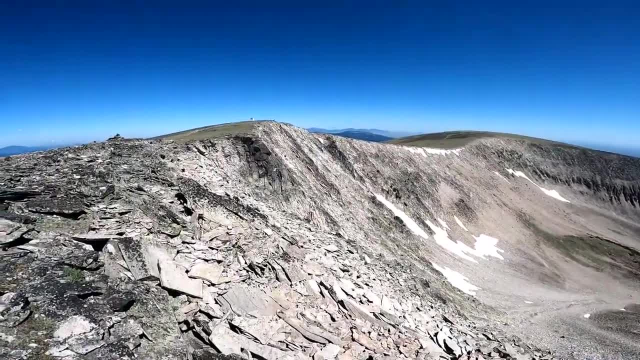 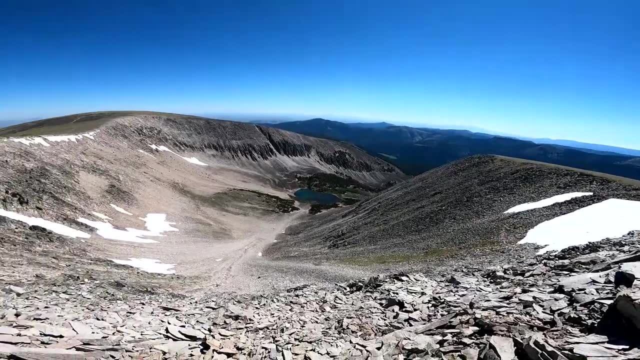 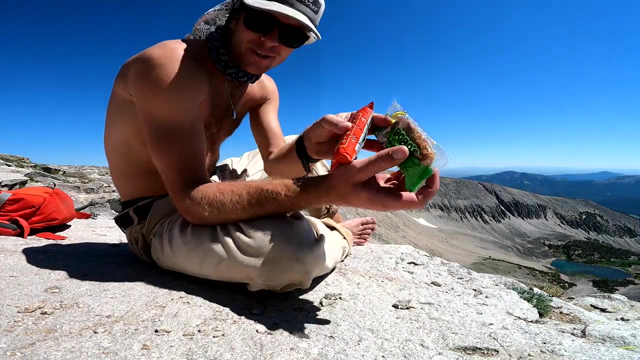 well, just coming over a final false Summit there. nice little Cirque up here. I wasn't really expecting this, to be honest, didn't know it cut off. I'm on the east side like this, but uh, Rhonda Lake down there. I saw on the map really nice, nice Ridge. two choices here for lunch: I've got the Bobo's. 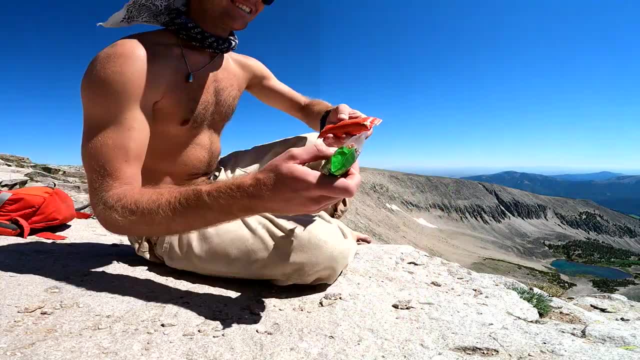 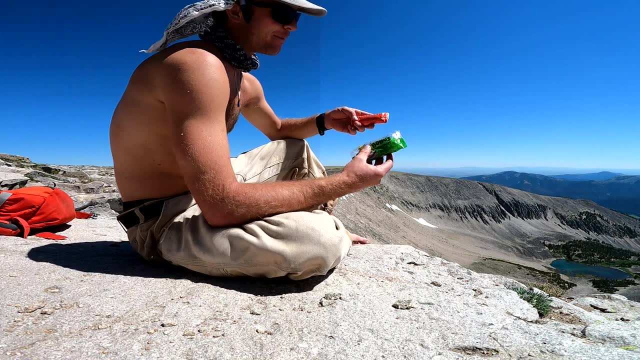 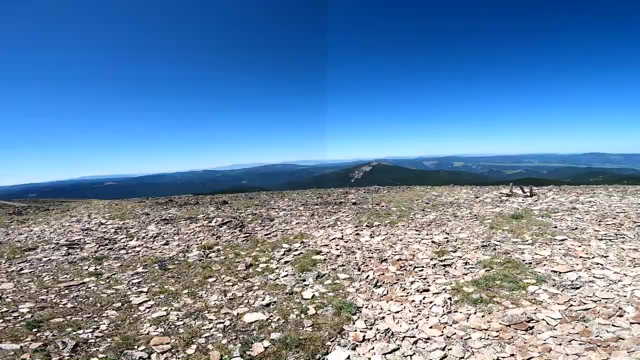 coconut or the larabar, which is inflated, uh, due to elevation gain, drop in the comments which is better, Bobo's larabar. I with both of them heavy and I'm going with Bobo's. I knew the whole time the rocks that I'm here interested in and and sampling, are these rocks right here you can kind? 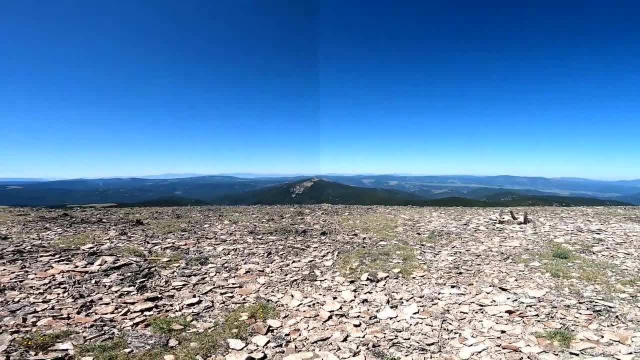 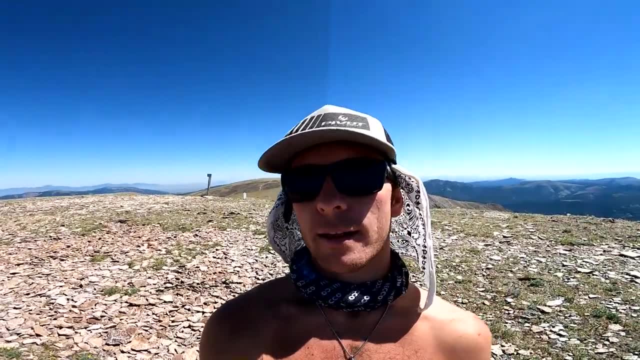 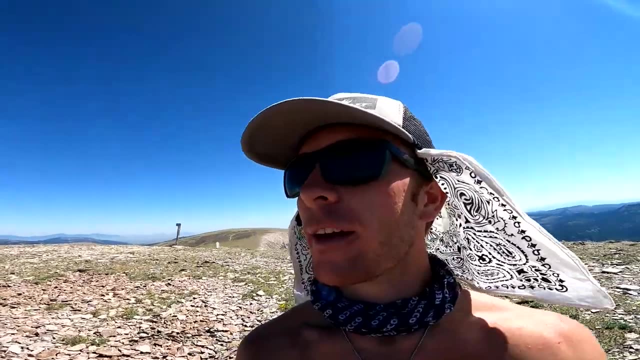 of see them outcropping over there. it's this big knob of paleoproterozoic granitic nice 1.8 billion year old basement rock that was exhumed from from depth um, and we're trying to figure out when that occurred. yeah, generally coming in here looking. uh, this was helpful to come up here, for sure, and I'm 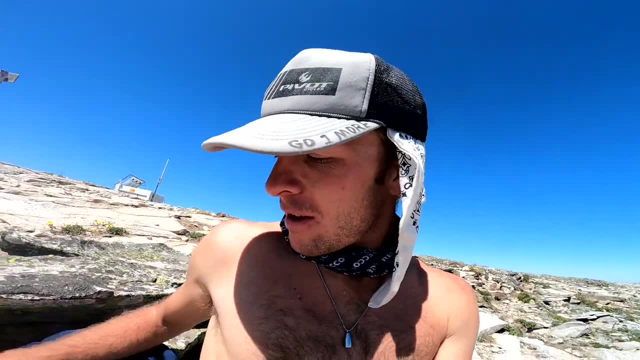 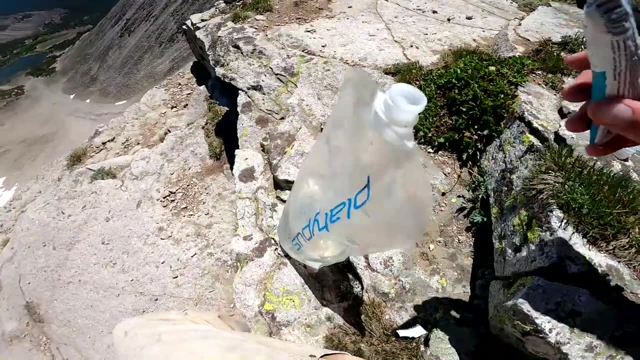 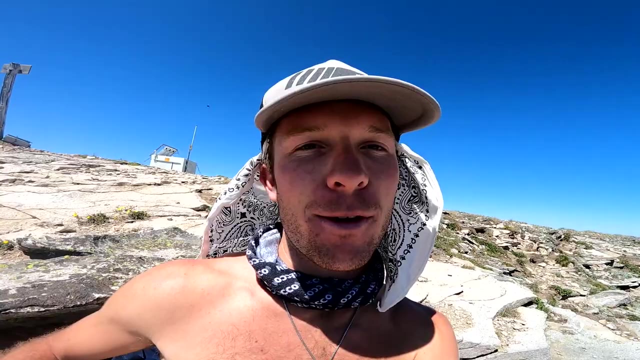 gonna. I'm gonna take some images that I can annotate. the plan now is to just bomb out of here and get to work on the rest of the day. not gonna do an update tour back at the truck check this out. second dose: baby liquid IV. sponsor me, I will rep your product proudly. electrolytes. out here, my clothes just. 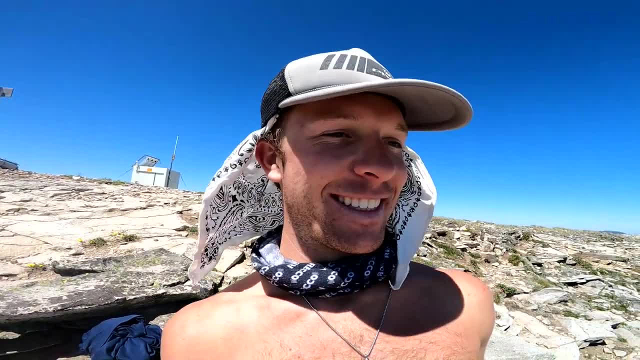 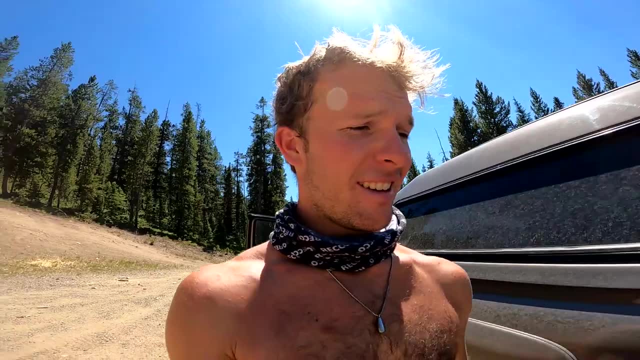 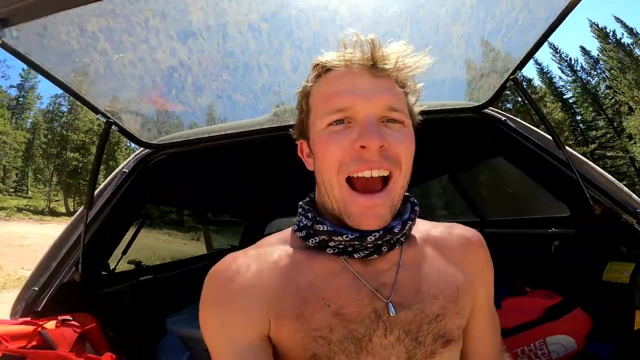 dried. I got sweaty as hell. that was kind of a gnarly uh hike up, honestly, but uh, it was definitely worth it. beautiful day. here we are back at the rig. um, made it off of the big Baldy Mountain, made it back, uh, back at the rig. now that was kind of a big effort, it uh. 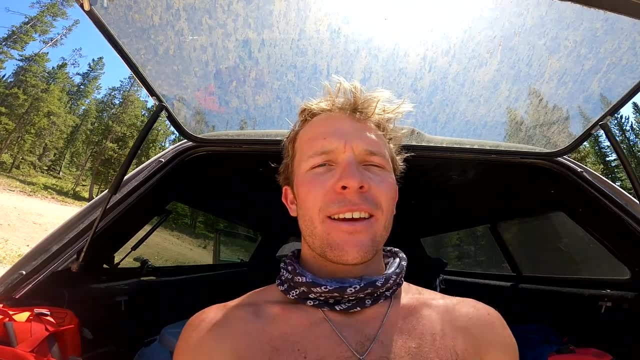 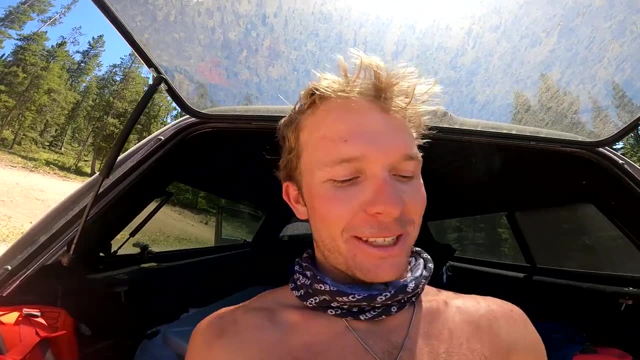 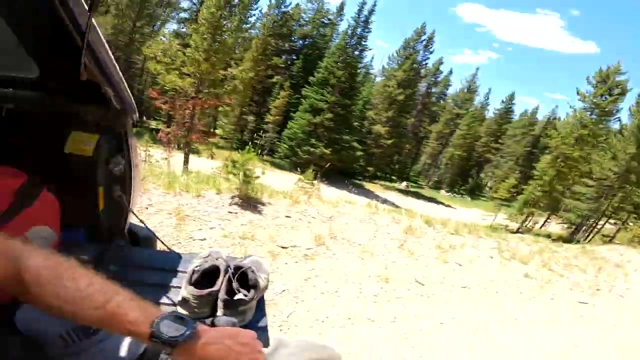 it ended up being a little longer than I was expecting, uh, but it was really doable. I just had to run out the last, like two or three miles, and I did it in the Carhartts, which is a true Savage mood, excuse me, true Savage move, running in these things, very uncomfortable, um, but yeah, you know. 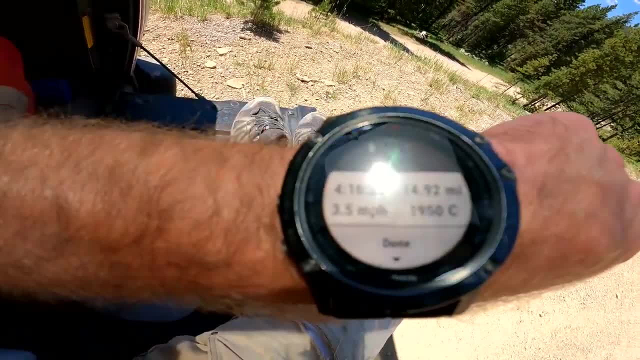 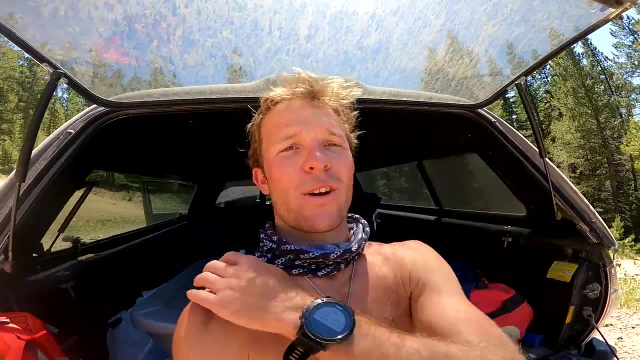 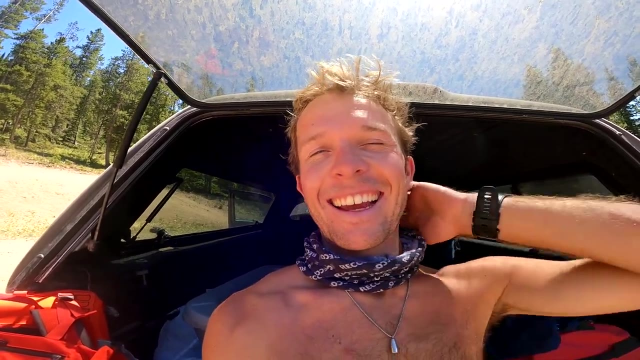 here's what we got. I don't know if you can see this. four hours 15 minutes, uh, 14.92 miles. so kind of fat, 100 feet of gain. man, now I'm gonna eat something I'm. I had that one bar and a couple liters of. 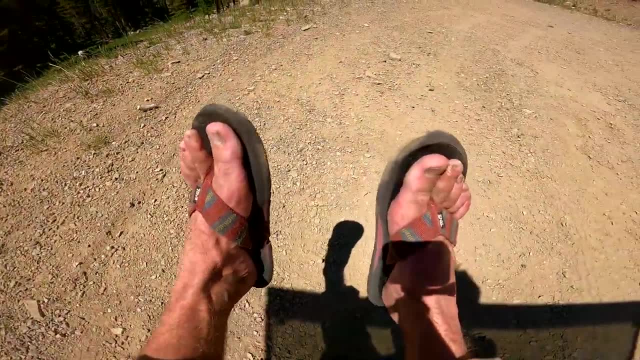 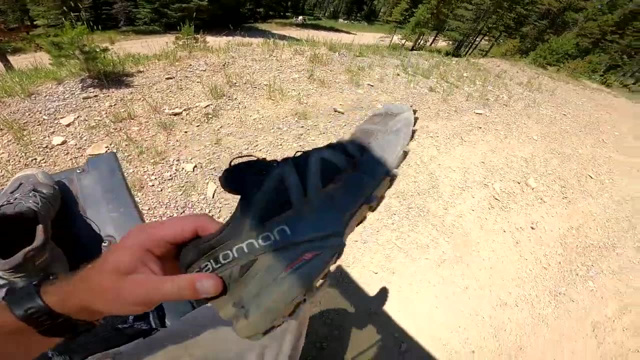 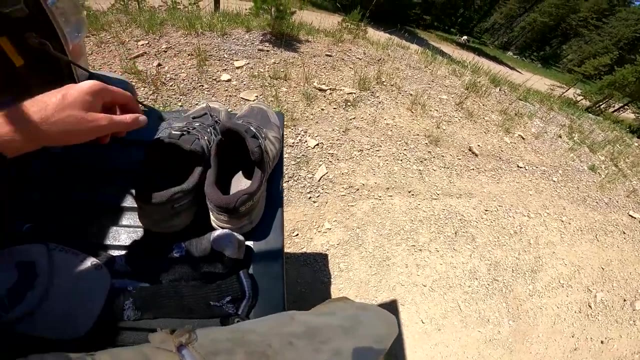 water so I need to chill for a sec for sure. feet not feeling too good. um these, I love these. I've always gotten these Solomon speed cross um, but these are completely gassed. they probably have like 400 miles on them of like hard miles, so my feet got thrashed also. I forgot to say I traded. 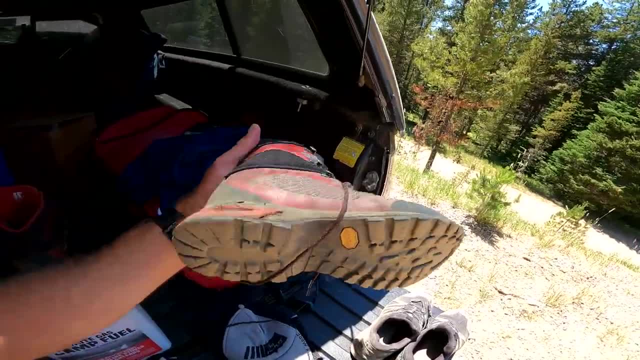 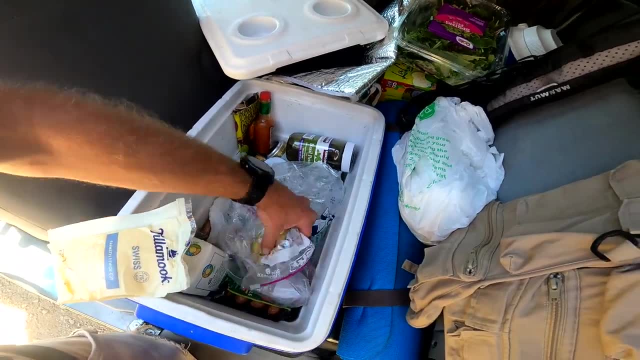 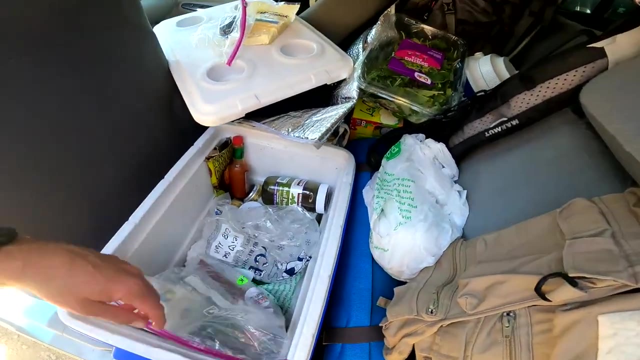 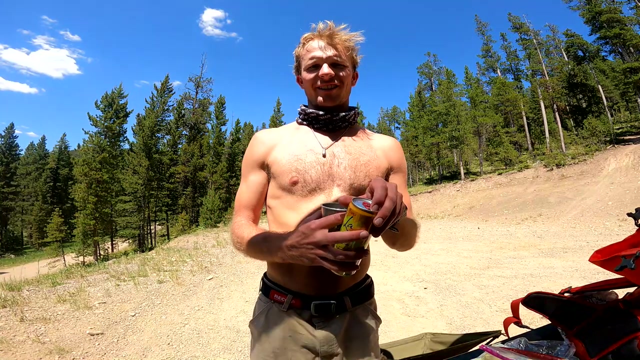 these out right after, right before I left. thank God I didn't wear my boots. I'm gonna go Swiss, ooh, nice and cold. half an avocado I have left, um, and then I don't. I don't often eat meat, but I'm in Montana and I was able to get some, uh, some elk. well, it's the simple things in life that make oh. 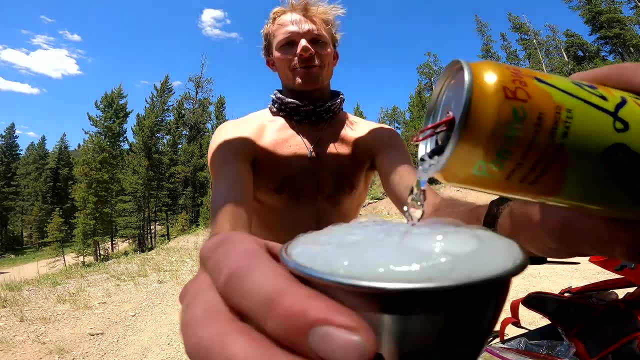 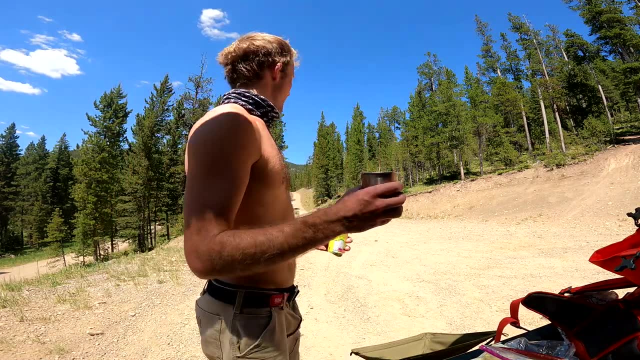 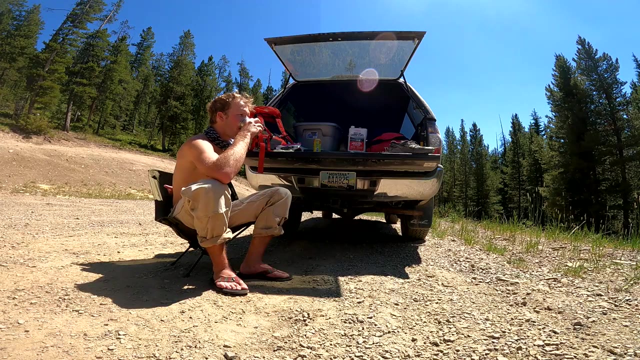 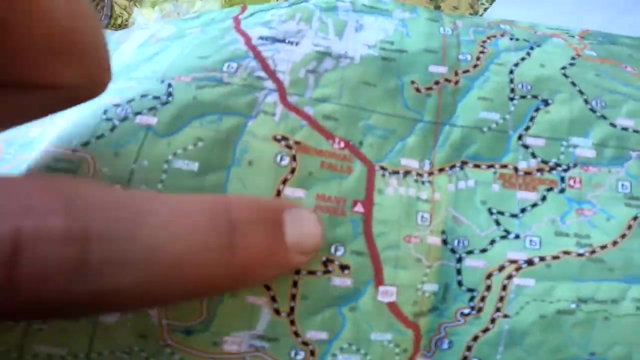 my God, you have no idea how good this sounds. look at that Crispy. that is a La Croix on ice. come across. ice out here is a delicacy, so we have lots of daylight left here. um, we're out here at Jefferson Creek. I'm gonna take it. 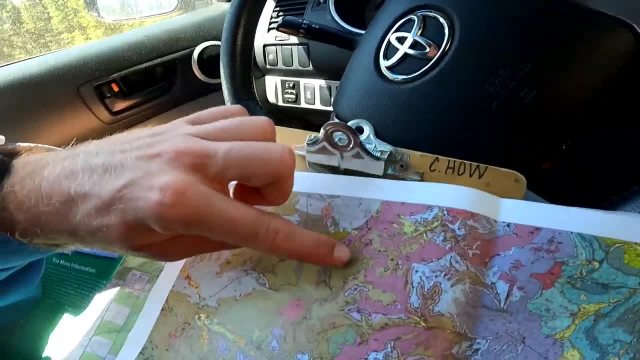 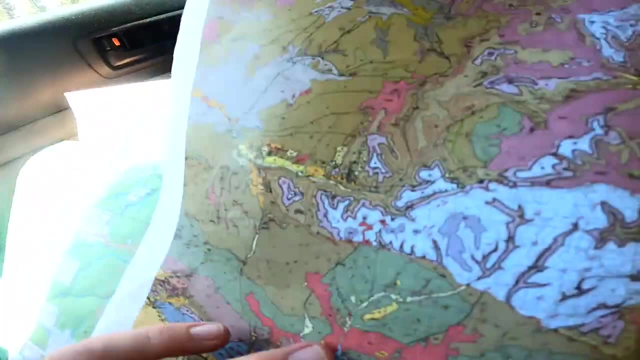 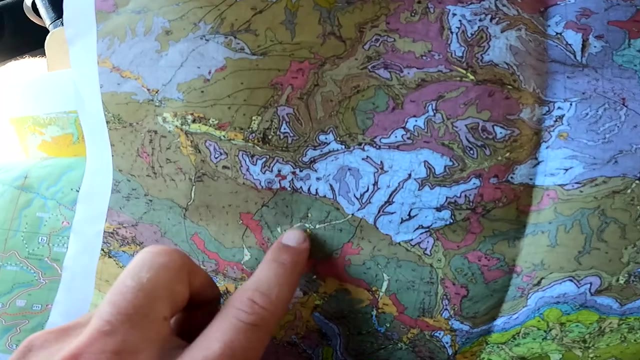 out to the highway and I'm gonna go south, so we're about right here. I want to wind all the way down to this, this structure that is very interesting to me. uh, this red line here. you can't really see it, but it separates these light blues and purples from the olives, um, and the dark greens. this is 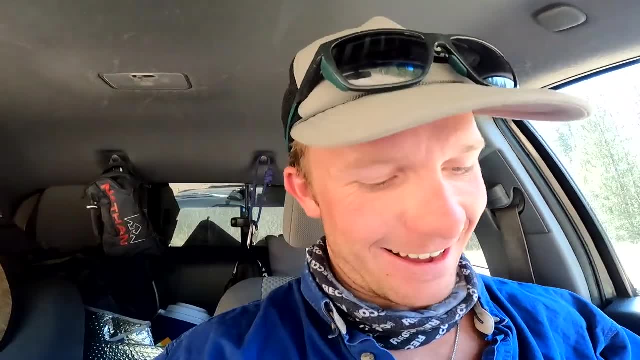 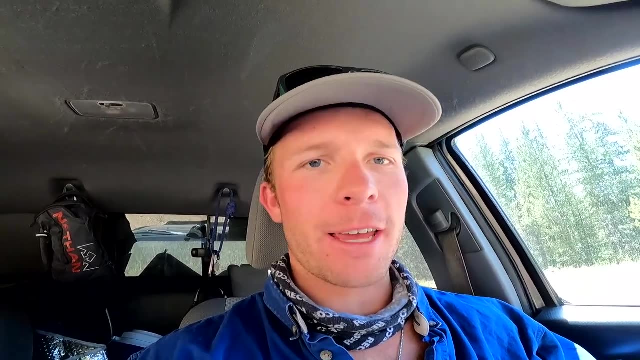 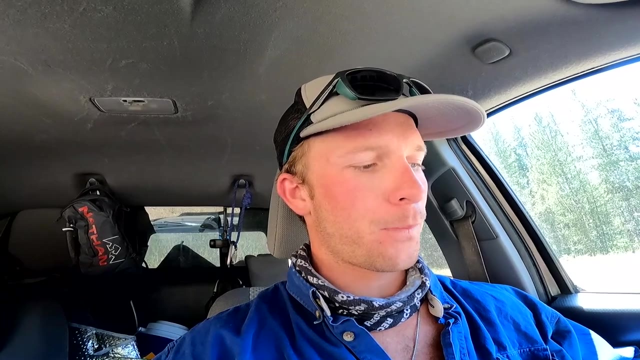 known as the volcano Valley fall. there's dubstep playing in the background. um this is an East West oriented fault, and on the map there are no indications of known kinematics, which means like there's no way to tell for sure which way um rock was being displaced. another thing that's uncertain is the kinematics, the kinematic history. 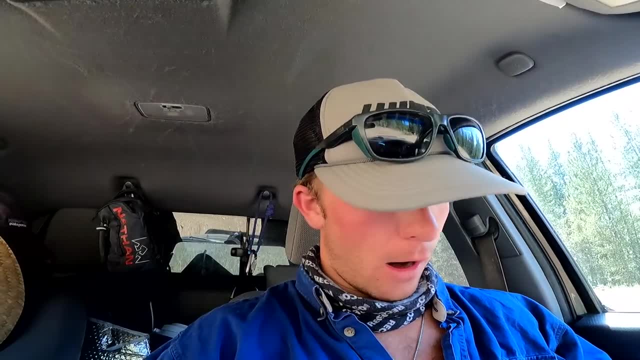 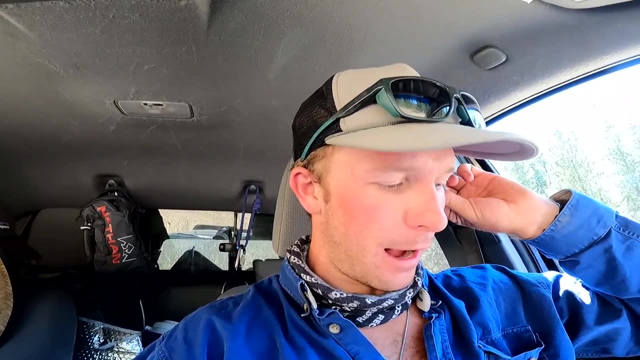 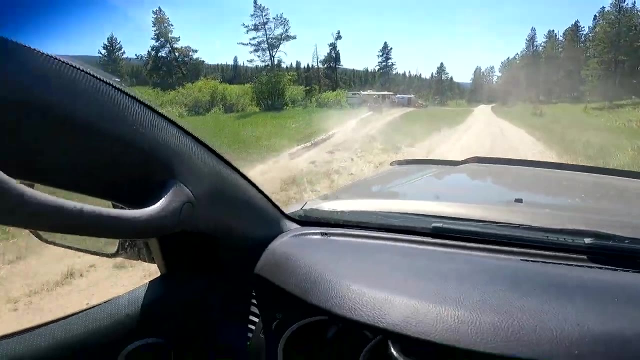 or when this fault was active. so I'm gonna head south- um, I might even bop into town really quick- which is a small little town, uh- to get some water and ice and nicotine, but primarily the first two things. look at this guy. he is, oh my God, dude, what a character. 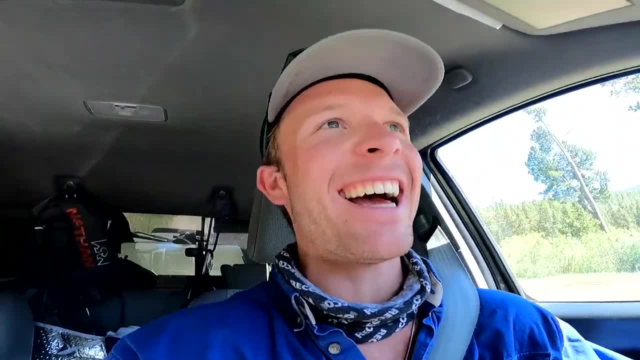 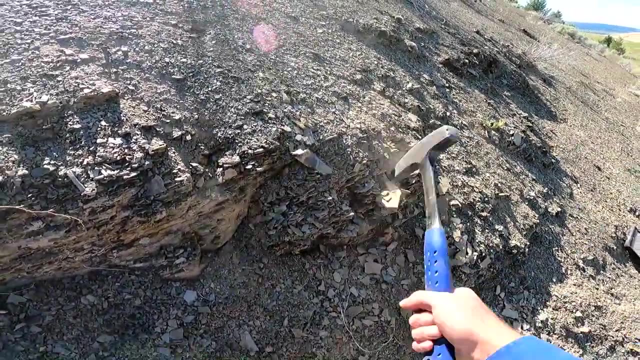 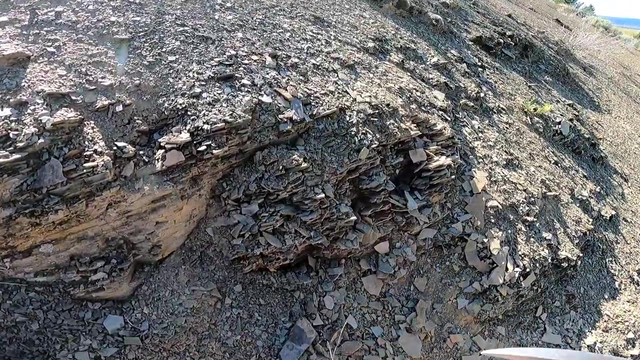 you know, we're just out here in Montana in the back roads. so here we are, new rock type, clearly not an igneous rock. this is, you know, at first glance what I would call a bluish red, finely laminated siltstone. this is actually called the Grayson. 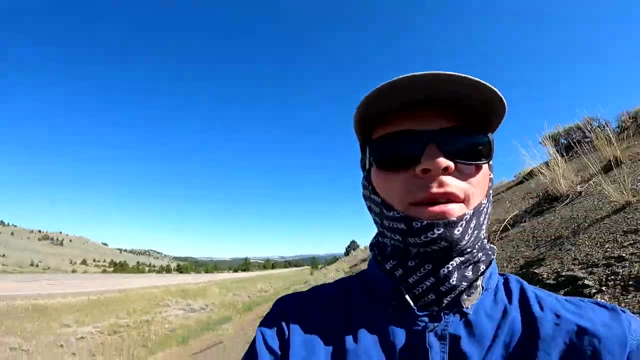 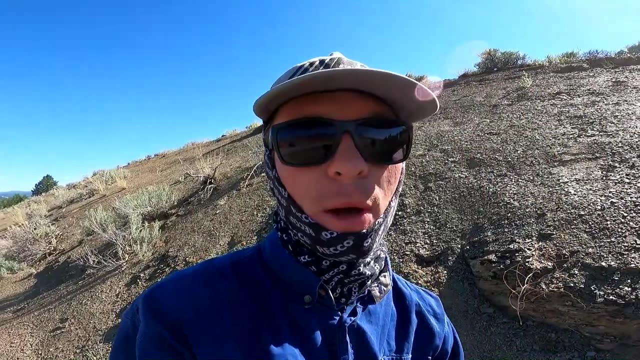 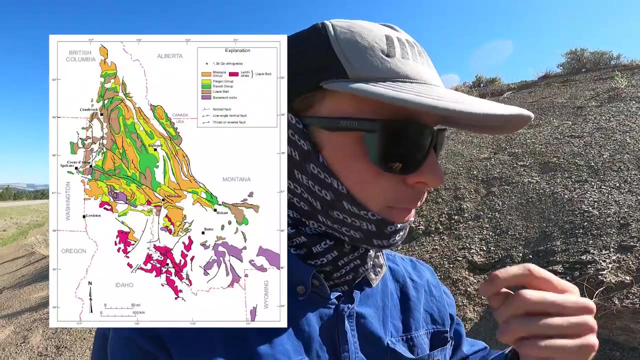 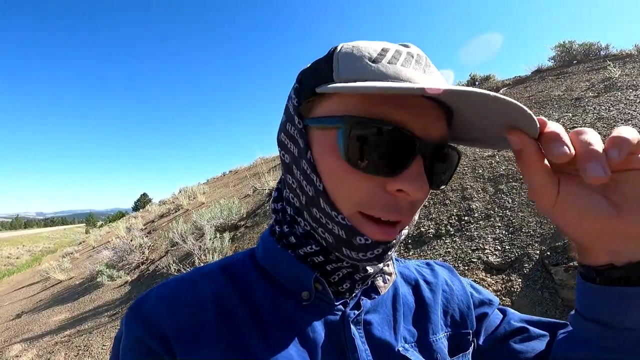 formation, um. it's the bottom, close to the bottom, of a? um gigantic stack of sedimentary Rock that we call the Belt super group, very extensive in Central down into Southwest Montana, um also very prevalent in Northwest Montana up into Canada. but this was basically in the mesoproterozoic. you know, over a billion years ago you had a lot of space that was. 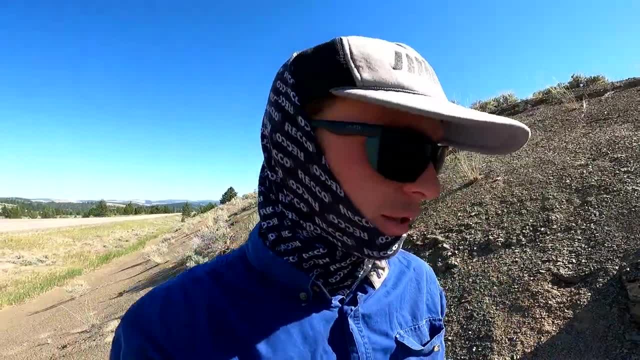 being made for these sediments to accumulate and later become sedimentary rocks. so I'm just taking some bedding measurements. um, it's about 7.5 feet long and then it's made of sediment, and that's what we're looking for in the belt super group. 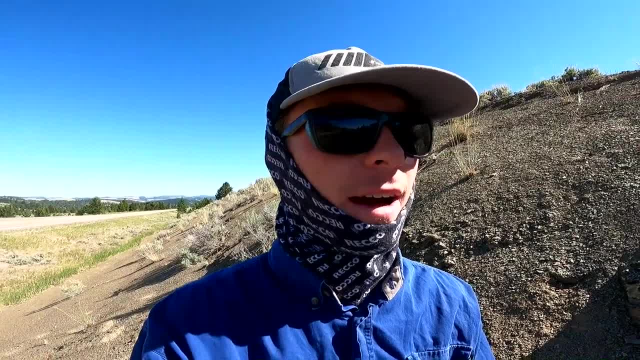 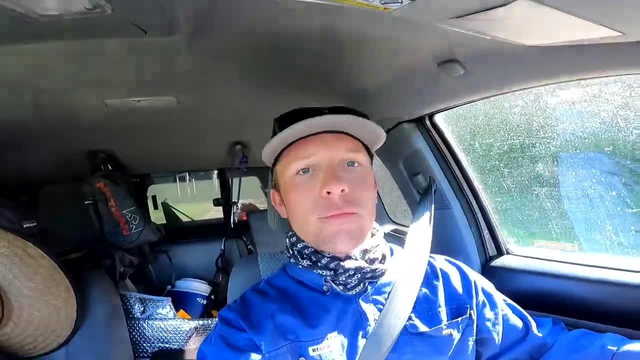 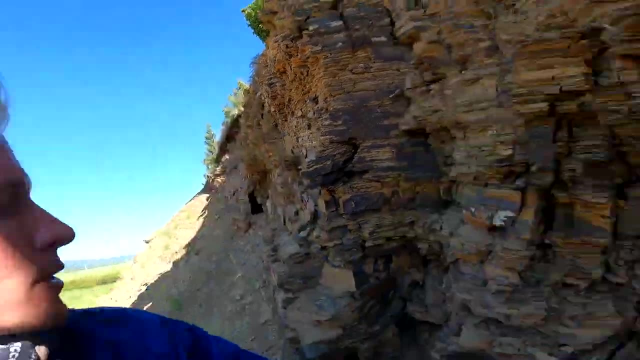 five pm, you know, and it's kind of the heat of the day, it's got to be about 85, 90 degrees, um. but wrapping up the day, looking at some belt stratigraphy, just wonderful. this is the, this is the newland formation, uh, which is stratigraphically below the grayson, which we 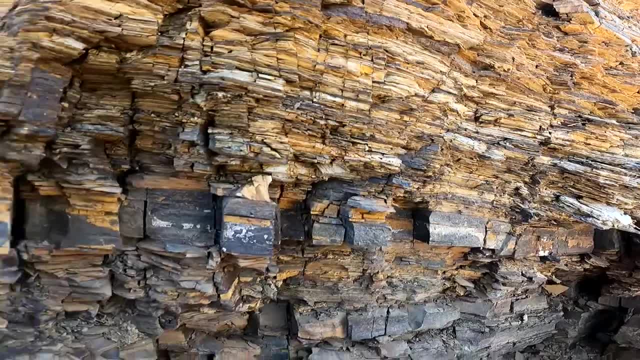 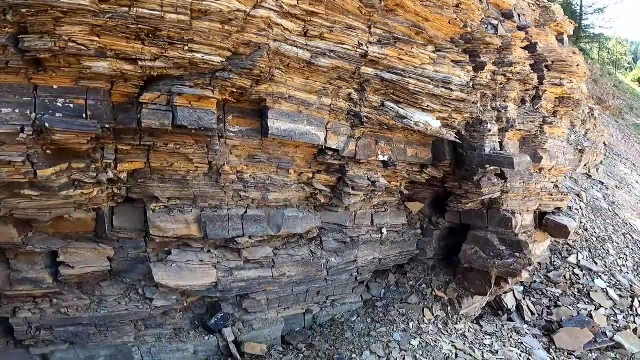 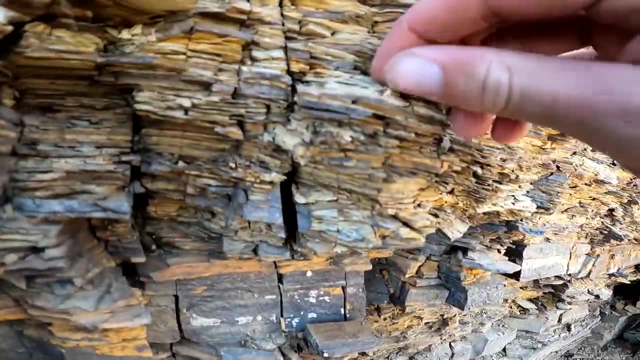 were just in kind of first order comparisons here. we certainly have some thicker beds. you know upwards of, you know five to ten, uh, maybe even yeah, i'd say five to ten centimeters in thickness. um, there's a lot more, uh, like interbedded clay stones, really fine grained. 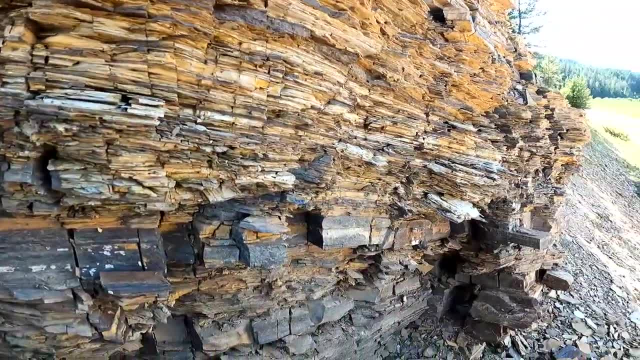 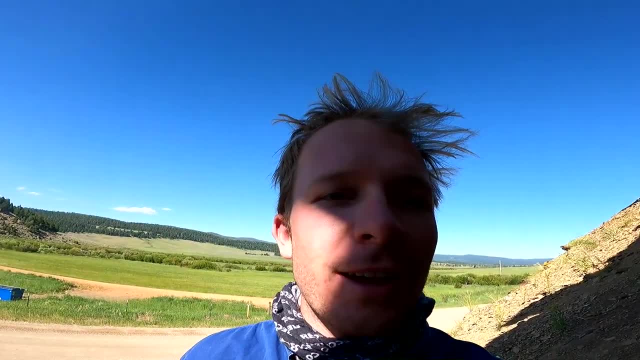 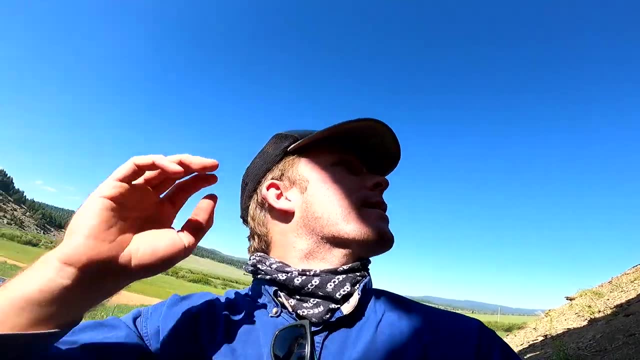 uh tend to be white. there's actually a trick for uh rubbing these types of rocks between your teeth to tell the difference between silt and clay, which i've done since i got here- delicious um, but yeah, i'm just uh gonna take some measurements at this outcrop and then might be the end of my geologizing. 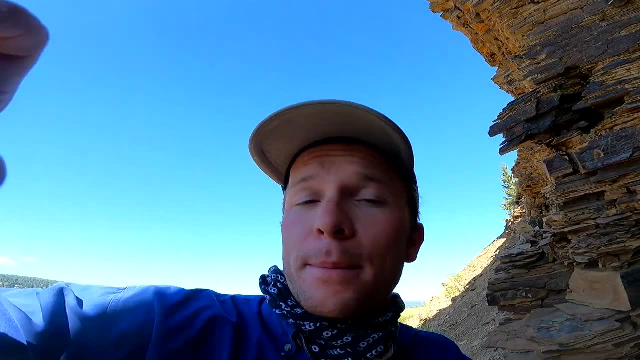 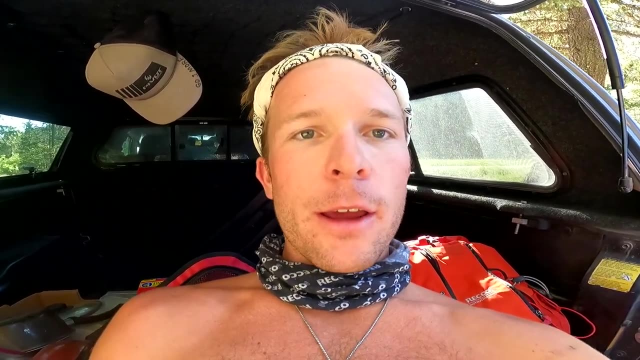 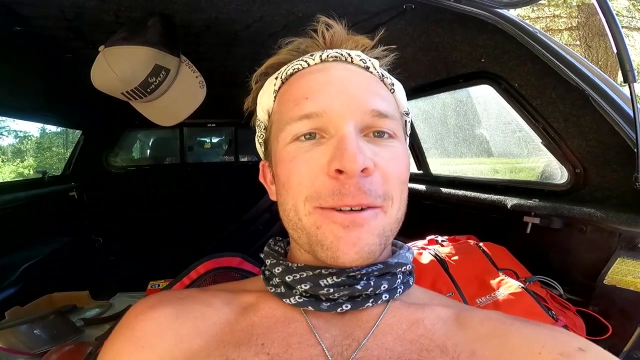 today. interesting stuff we'll see at the camp. all right, everyone, i have a little camp established here. uh, it's about 6: 30 in the evening, the sun doesn't set for a while. but i've got some things i can do and now is my favorite time of the day and that is the daily swim in the creek or lake or whatever. 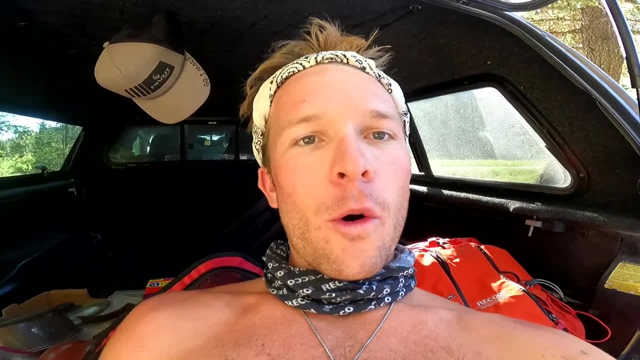 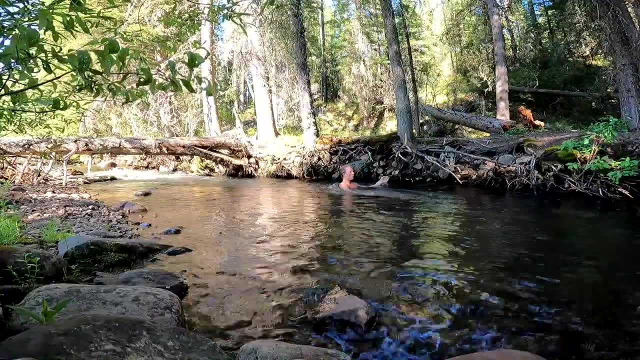 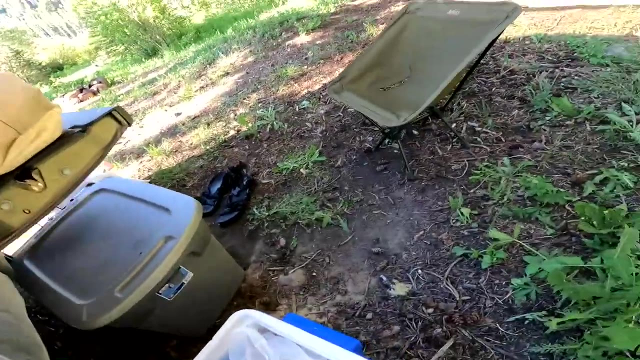 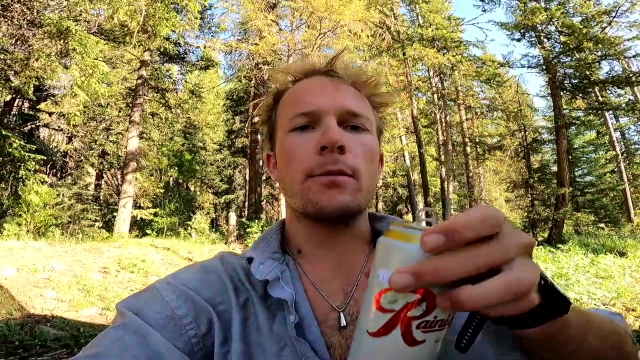 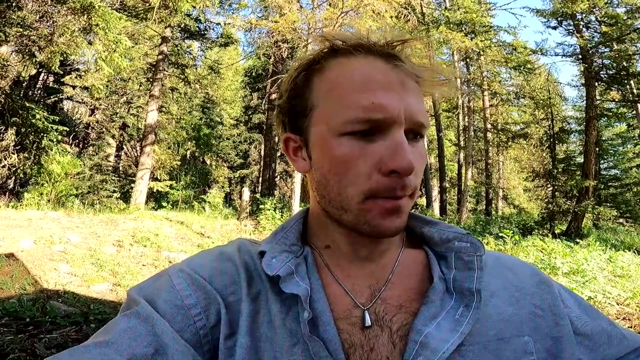 is nearby. i'm about to go get in some cold water and it's going to feel amazing. always my favorite wham, all right. so i had a little swim and i'm gonna enjoy a cold beer. you know, by the creek here i'd say it's earned today. um, you know, there are some days that are. 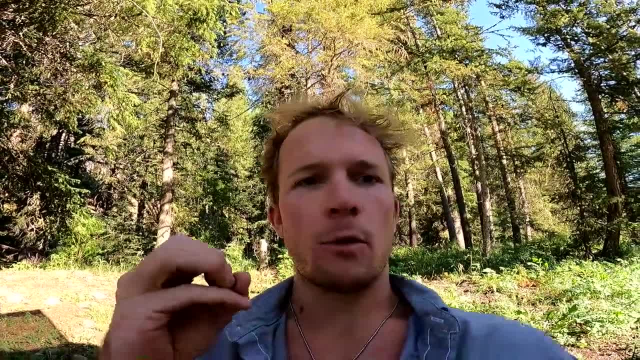 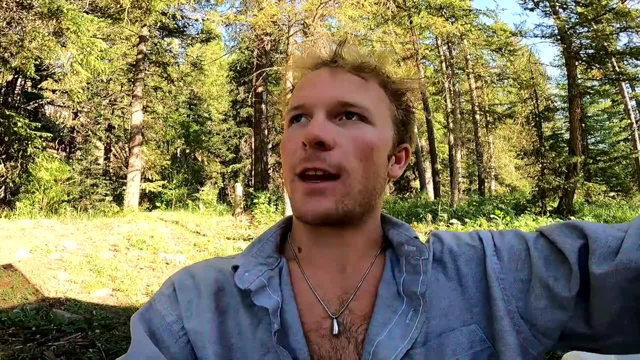 much more detail oriented, uh, much more localized and taking, you know, detailed measurements and detailed notes. today it was pretty fun to just kind of go send it and go look at some from some different viewpoints and then did see some geology at the end of the day, and so i think 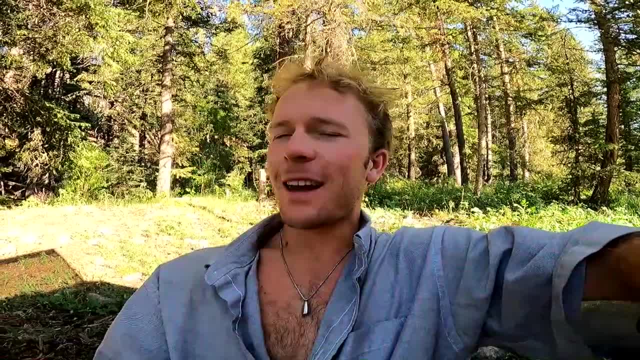 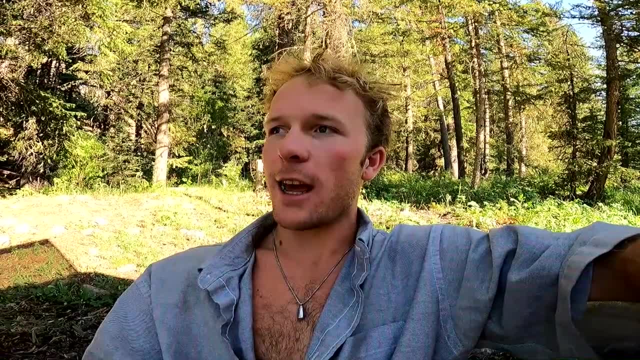 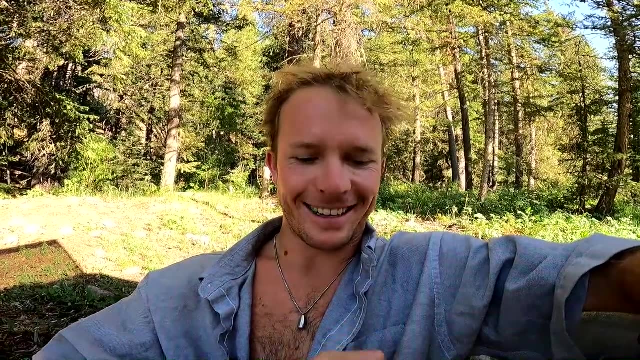 i deserve a beer. i'm justifying it. it's almost felt like I've had someone with me today, So this has been fun. Um, but this really is how it is daily And I prefer not filming it. Um, I have lotion on my hand. I prefer not filming it because it doesn't really feel right to. 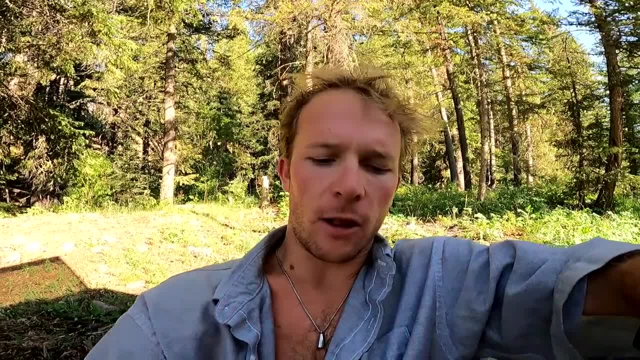 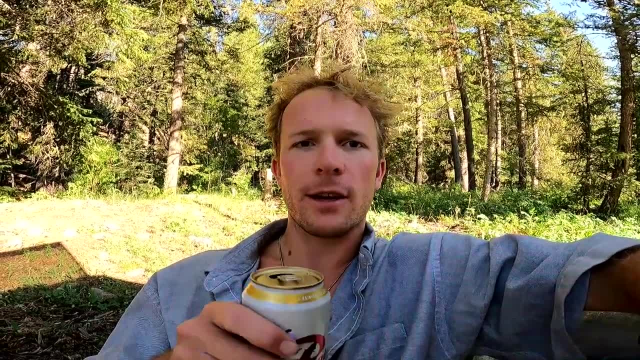 it kind of takes you out of nature to some extent. but I do this a lot, So I figured it would be fun to share the experience with you And, um yeah, we'll see at dinnertime. Then I'll just check off. 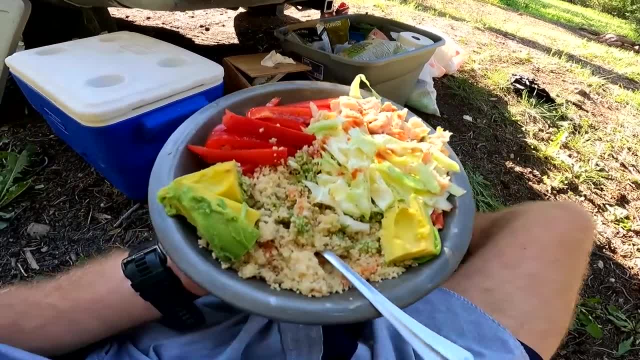 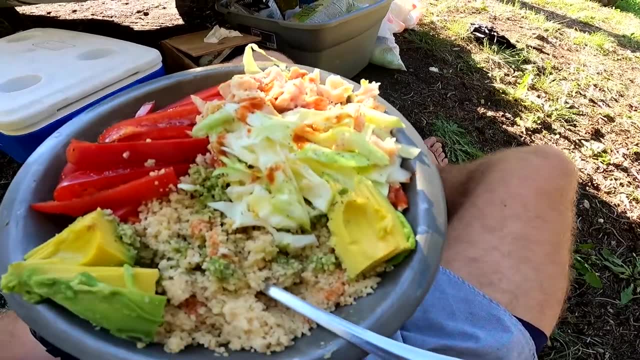 for the night. Pretty easy, We've got, uh, couscous with pesto, half an avocado, some fresh bell pepper, um, a little bit of greenery with some tuna, olive oil, salt pepper, hot sauce. 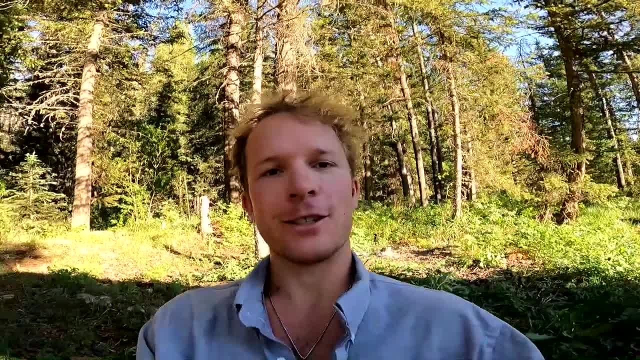 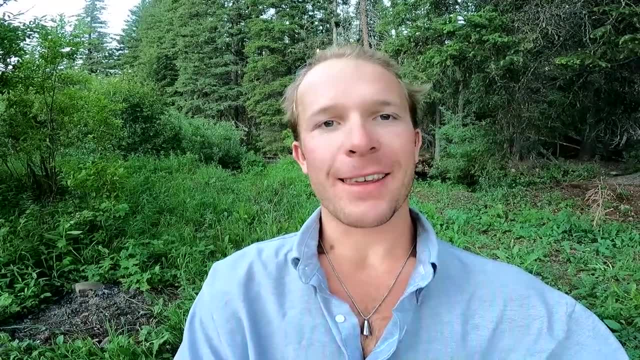 Very simple. Just got to get all the nutrients you can get out here, Alrighty. Hey everybody. This is goodbye for the day. A beautiful Wednesday in the wilderness of Montana. I hope you enjoyed coming along for the ride. I'm going to go back to silence tomorrow.